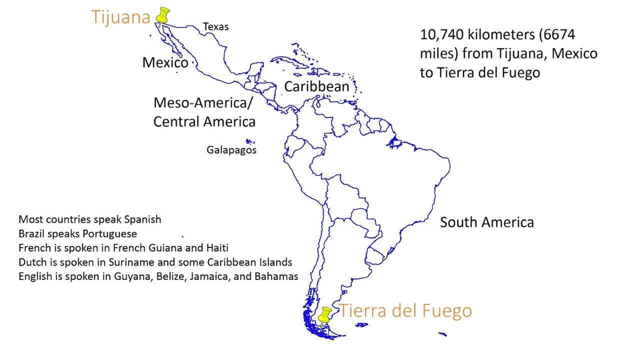 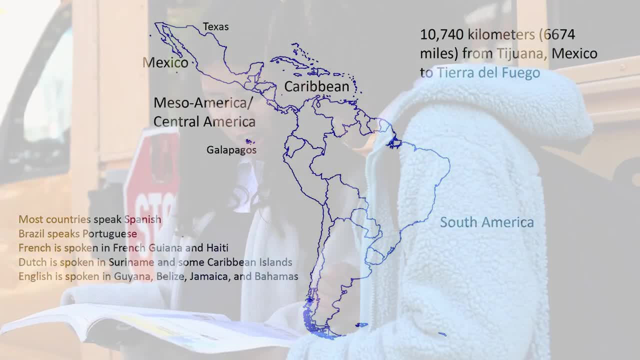 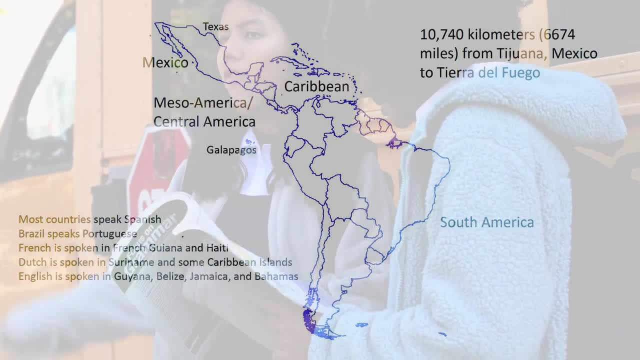 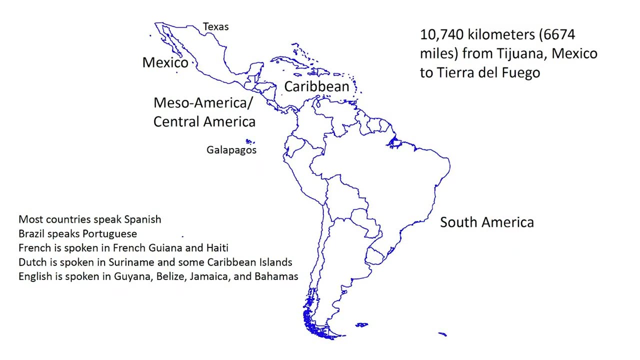 attract more Hispanic and Latinx students to be interested in learning about Latin America. Many organizations and disciplines, including our own, recognize the importance of increasing diversity in science and we think that teaching about Latin America is a good way to engage Hispanic and Latinx students to want to learn more. Second, we think that non-Hispanic 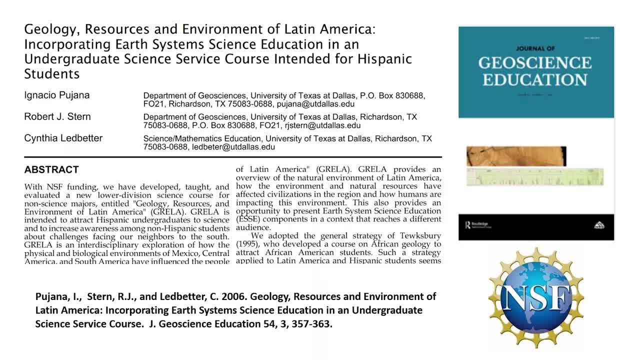 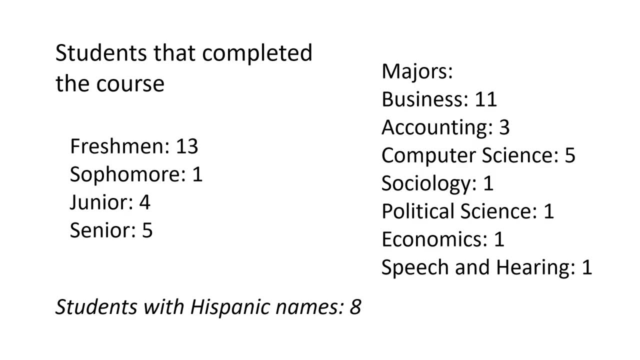 students need to learn more about the lands to the south. For this purpose, we updated a course we developed with NSF support in the 1990s and taught this to 23 students in fall of 2021.. The class attracted mostly freshmen, No science majors enrolled, and 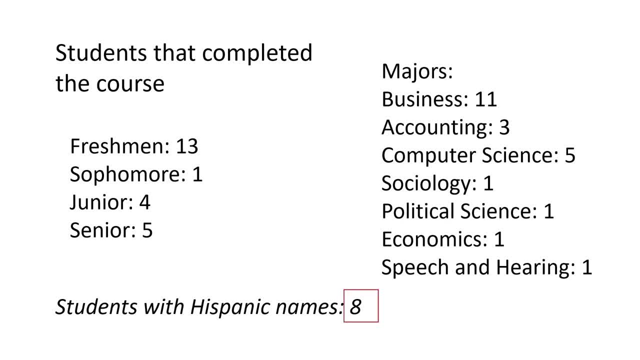 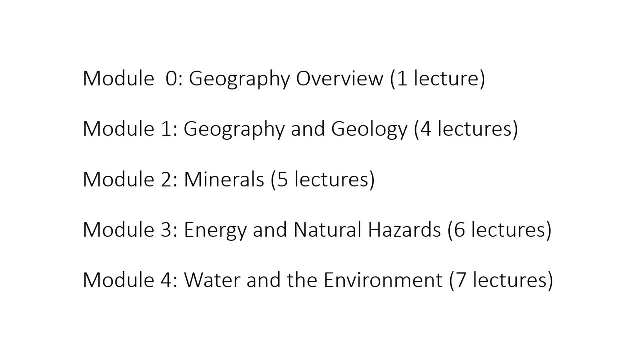 there were eight students with Hispanic last names. There's no suitable textbook, so course content is based on 23 lectures that are grouped into five modules: Geography and Geology, Minerals, Energy and Natural Hazards, and Water and the Environment. Because it is so important that 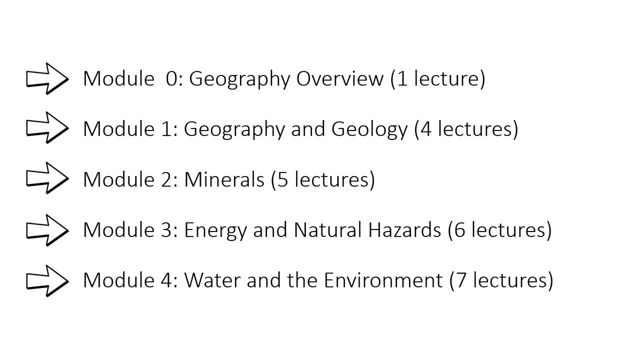 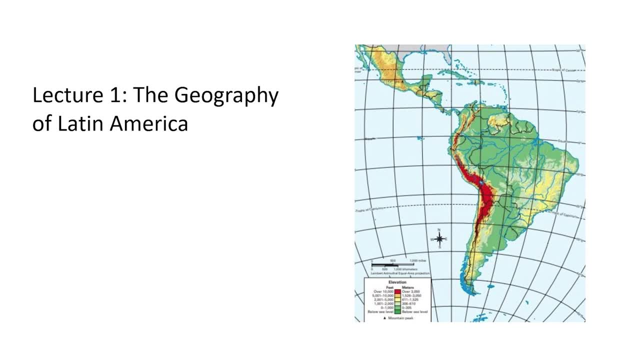 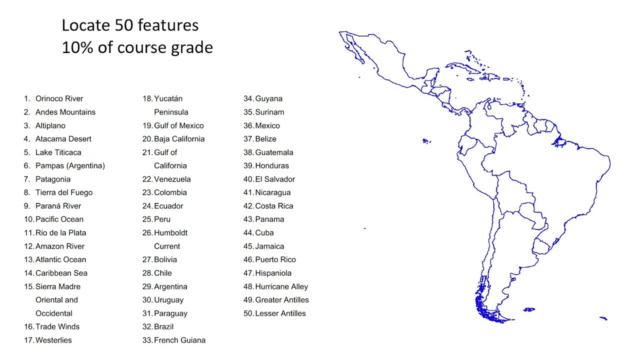 students grasp where things are. the course begins with a lecture on the geography of Latin America: its regions, nations and important physical features, followed by a test over this material. There are no surprises in the test. The students know which features they will be asked to name. 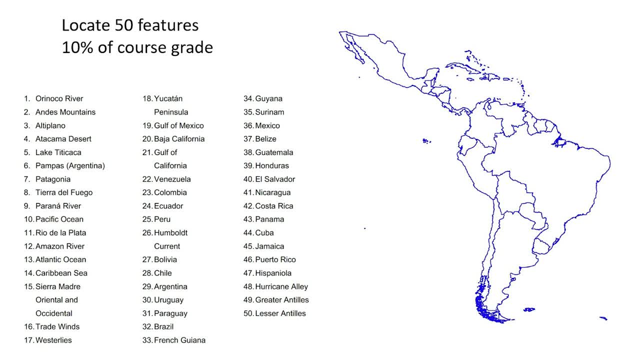 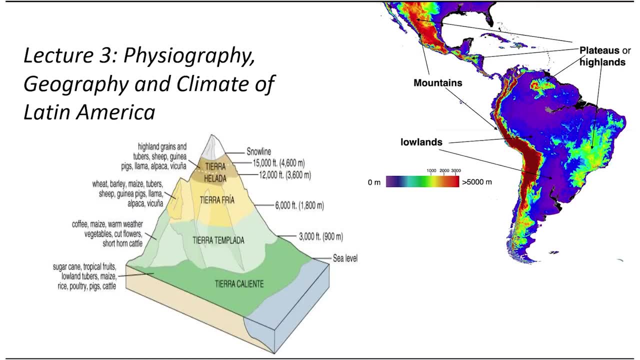 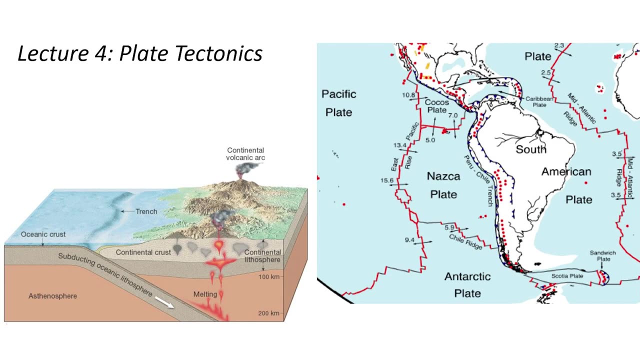 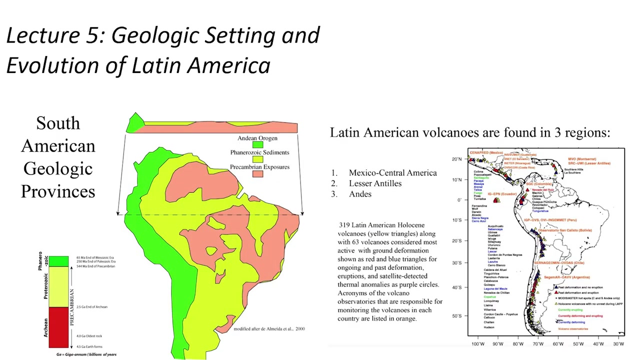 and are given a few days to study. The next four lectures are based on the geography and then its physical geography. Because the course is aimed at non-science majors, this module is finished by lectures that introduce plate tectonic concepts and outline the geologic evolution of Latin America. 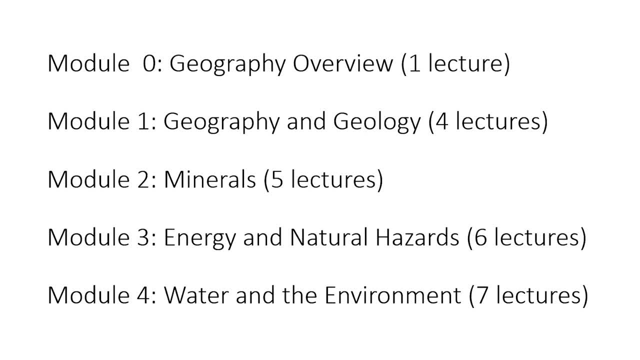 The next five lectures comprise the second course module, focused on mining and minerals. This module also allows students to study the geological evolution of Latin America. The next five lectures comprise the second course module, focused on mining and minerals. This module also allows us to briefly review the early history of Latin America. The first lecture explores how and when. 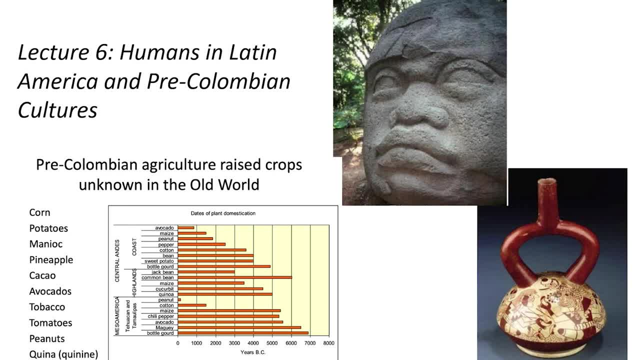 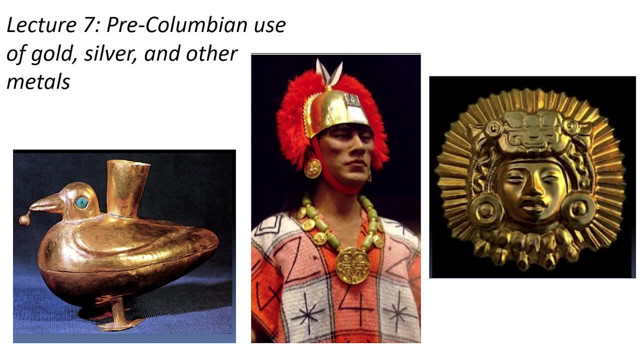 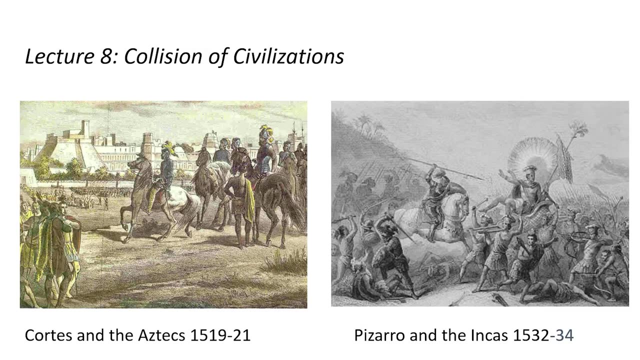 people came to the region, leading to the great Inca and Aztec civilizations. Next we discuss how metals were used by pre-Columbian people. This leads us naturally to the Spanish conquest of the Aztecs and the Incas- the collision of civilizations, and then to a lecture on how a special 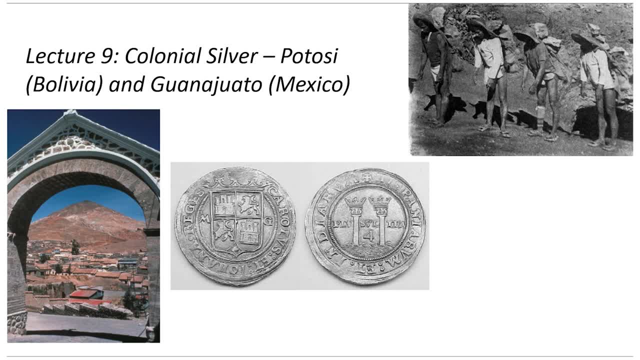 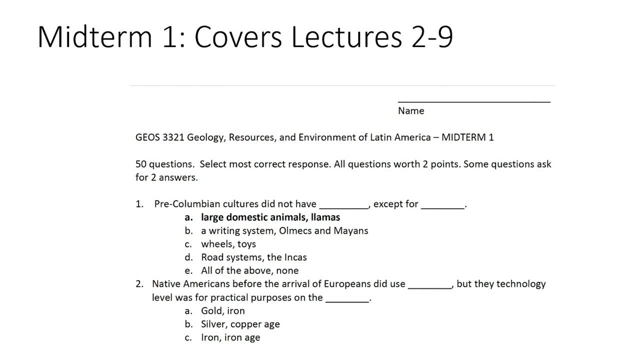 resource, especially silver mining, dominated the colonial economies of Mexico and Peru. These eight lectures are followed by the first midterm motivating students to review their notes and the slide decks which we post online. We correct the midterm quickly and go over right answers in the next class. 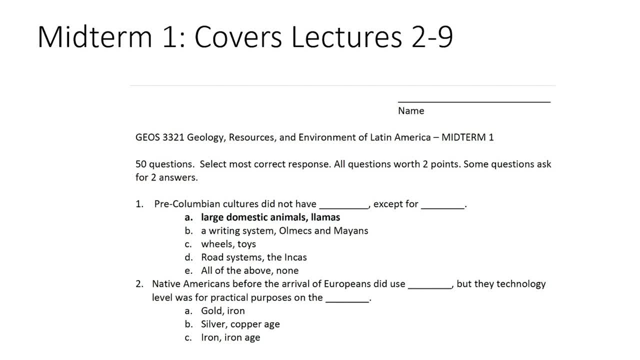 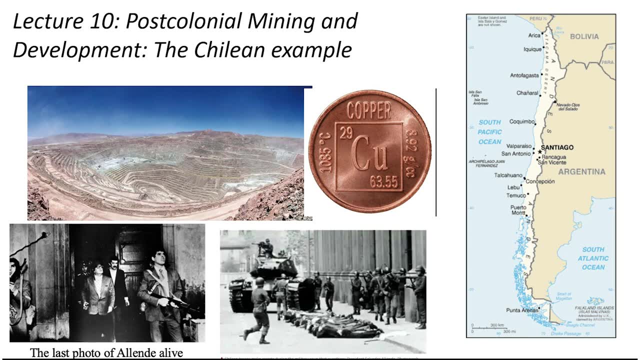 before giving the last lecture in the Minerals and Mining module, which explores nitrate and copper mining in the Atacama Desert of northern Chile. which explores nitrate and copper mining in the Atacama Desert of northern Chile and how exploitation of these deposits led to a 19th century war and a 20th century military coup. 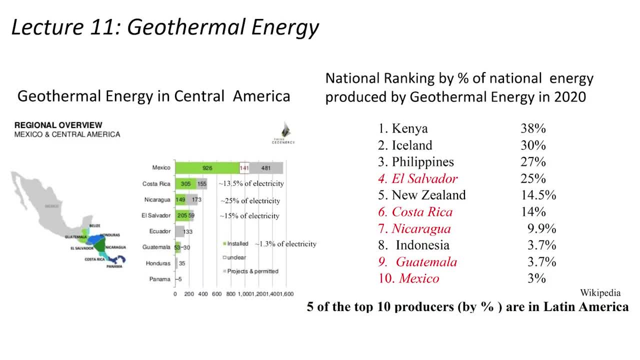 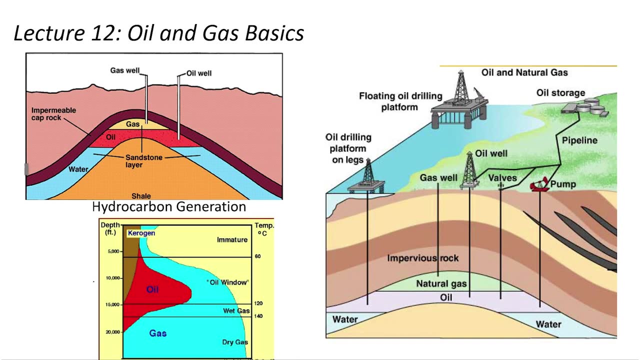 The next module is an Overview of Latin American Energy and Natural Hazards. This begins with an explanation of geothermal energy, which is especially important for Mexico and Central America. Next, we devote two lectures to oil and gas. The first provides some basic information about how oil and natural gas all work together. 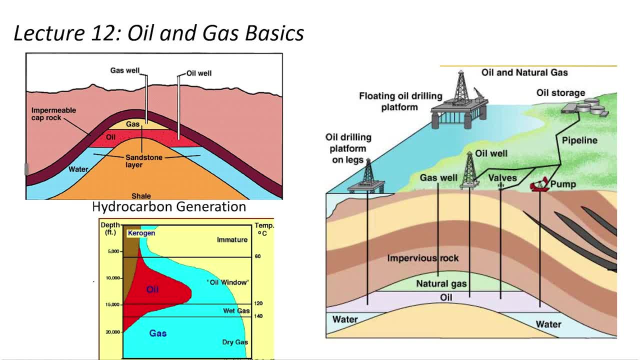 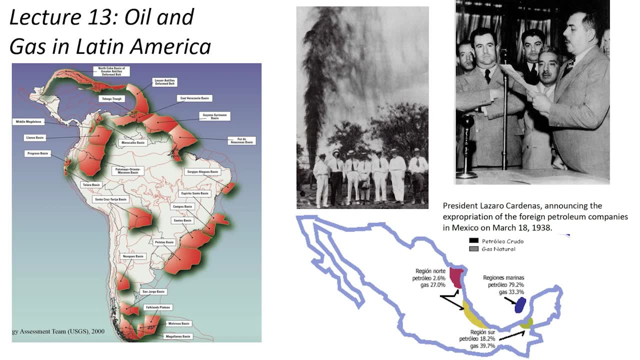 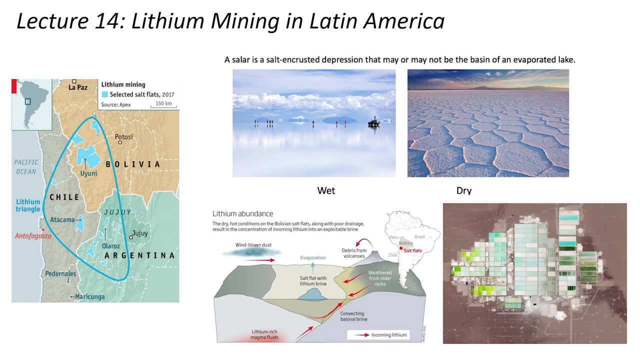 natural gas form and where it is found. and the second discusses where it is found in Latin America and some history about how these deposits were discovered and how these have affected the region's development. The next lecture focuses on increasingly important deposits of lithium needed for powering electric. 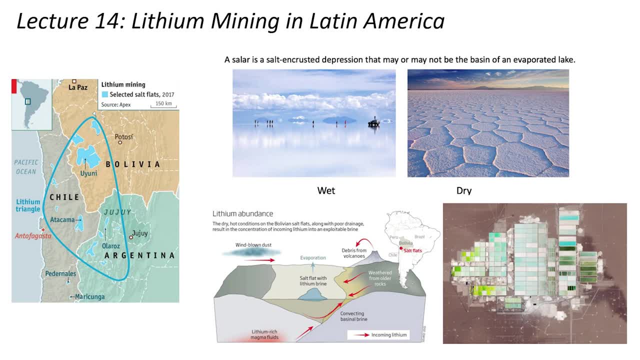 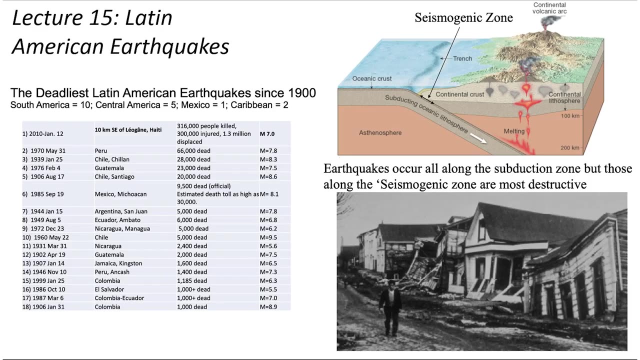 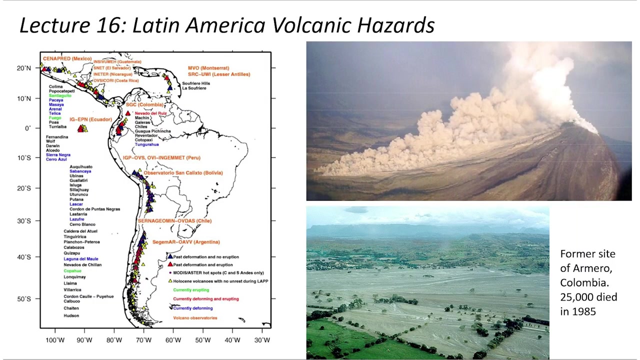 cars and battery storage of electricity generated from the sun and the wind. Mining dry lake beds or salars for lithium is causing environmental concerns and political unrest. The exploration of Latin American energy is followed by two lectures on natural hazards, first about earthquakes and then about volcanic eruptions, both of which are related to the. 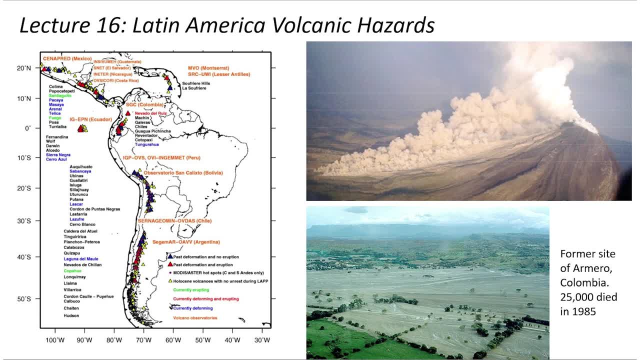 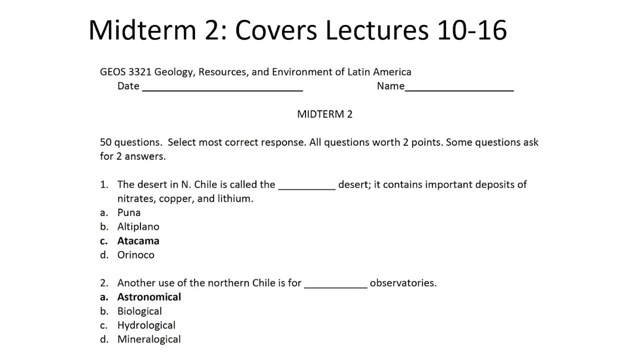 plate tectonic setting of Latin America. completing the second course module. This is followed by the second midterm, Again motivating students, We correct the midterm quickly and go over the right answers in the next class. before beginning seven lectures of the last module on water and the environment. 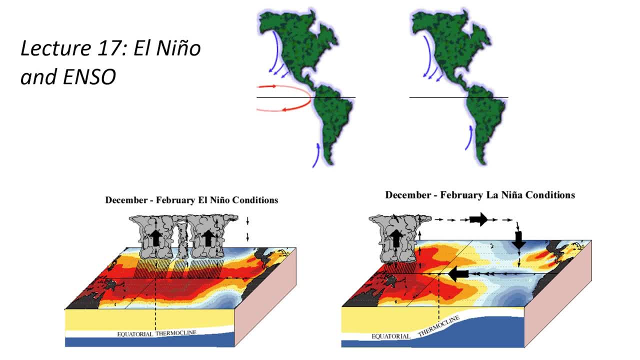 First is a lecture on the coupled oceanographic atmospheric phenomena called El Niño, which is also known as the El Niño Southern Oscillation or ENSOGL. This lecture also lets us explore the link between the trade winds, Ocean currents, nutrient supply and the marine food chain. 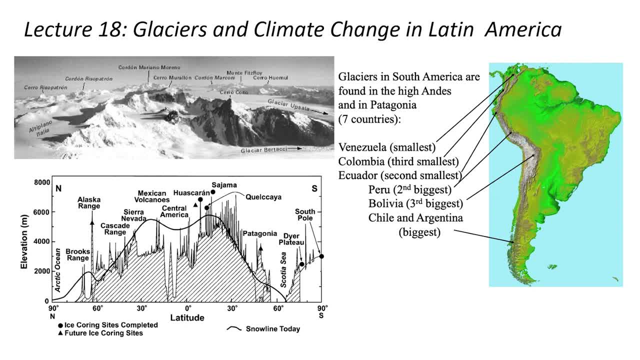 Next is a lecture about the glaciers of Latin America. Alpine glaciers near the equator are particularly interesting because they preserve an excellent climate record that is rapidly disappearing due to global climate change, hurting especially nearby farmers who rely on glacial meltwater for their crops. 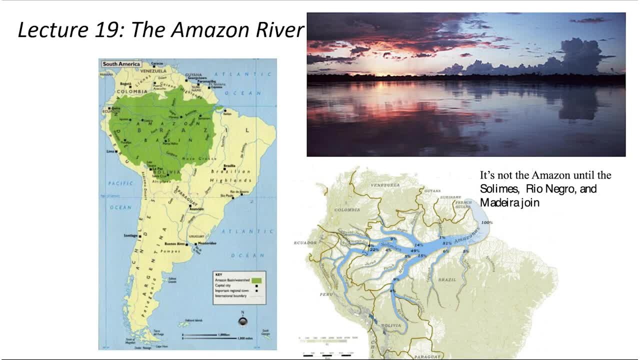 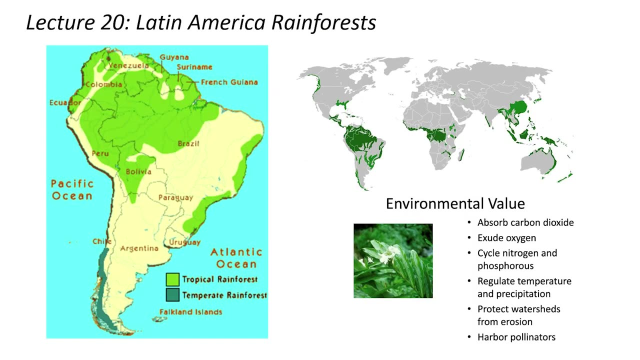 A lecture about. the Amazon River is next By far the biggest river in the world. We discuss not only the river system itself, but also explain why it is so large and outline some of the remarkable animals and plants that depend on it. Following Naturally after this, we lecture about Latin American rainforests, especially 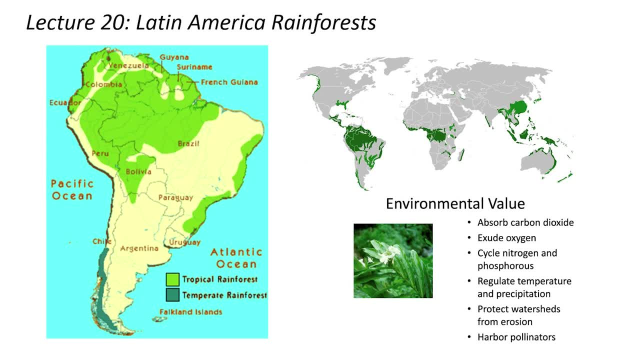 but not exclusively about the Amazon rainforest. We explore a number of topics, including the climate required to produce rainforests and their trophic systems and animals. We also explain why rainforests are important And outline how these are being reduced in size. 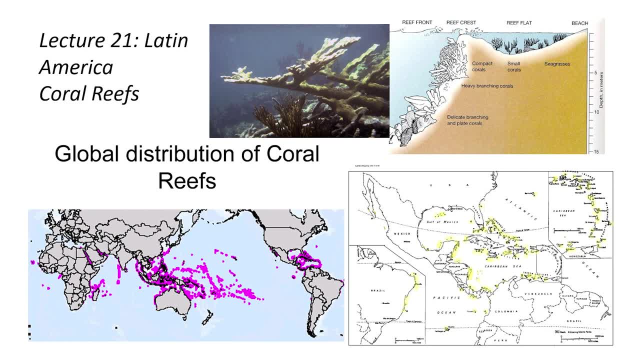 The next lecture explores the coral reefs of Latin America, which are concentrated around the Caribbean. We explain that coral reefs are remarkable examples of symbiosis with photosynthetic algae living in soft tissues of the coral animal host, and how global warming causes the algae to leave, leading to coral death and bleaching. 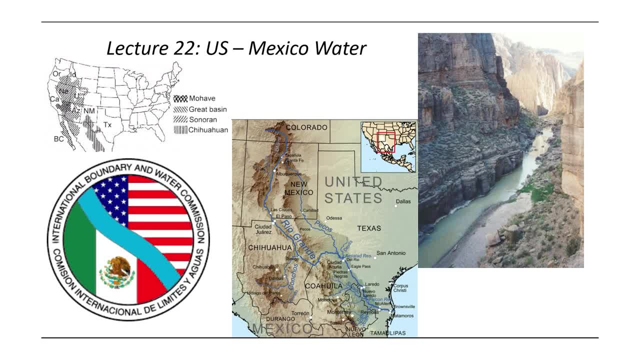 The next two lectures explore things closer to the ocean. The next two lectures explore things closer to the ocean. The next two lectures explore things closer to the ocean And the first two lectures explore things closer to the United States, first discussing the challenges of sharing the limited water of the Rio Grande and Rio Conchos, which flow 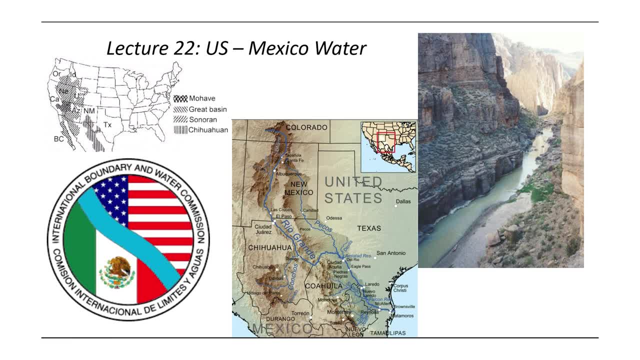 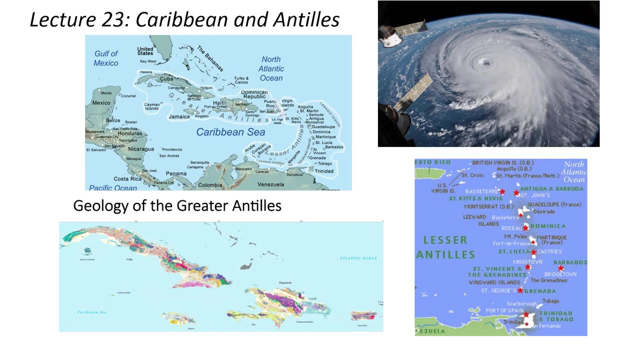 through the Chihuahuan desert between the United States and Mexico. We explore how population growth in this region is stressing water supplies and the importance of treaties and bilateral monitoring agencies for sharing this scarce resource between the two nations. The final lecture is an overview of the Antilles, where the people of Tuenதي and the Antilles 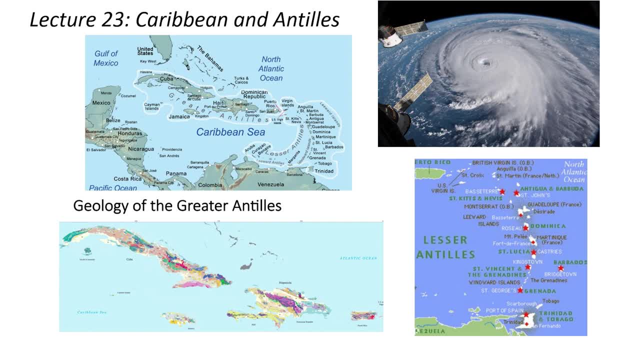 were located at the beginning of the Cretaceous period in the Aegean Sea. And the last one is an overview of the Antilles, where the people of Tuyetl, mujeres, of the Antilles, 12 nations and 19 dependencies live on many islands on the north, south and east rim. 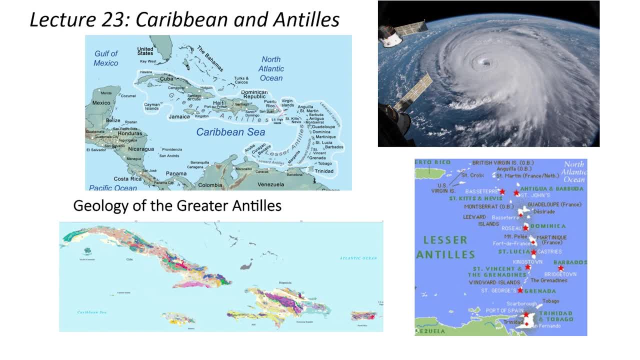 of the Caribbean Sea. Many people do not consider this region as part of Latin America, but we think it deserves to be included as part of the course. This is followed by the third midterm, again motivating students to review their notes and the slide decks. 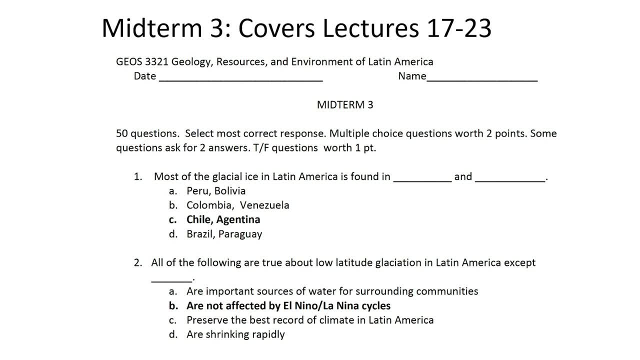 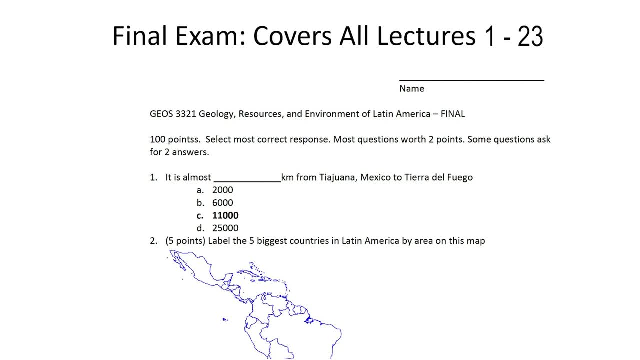 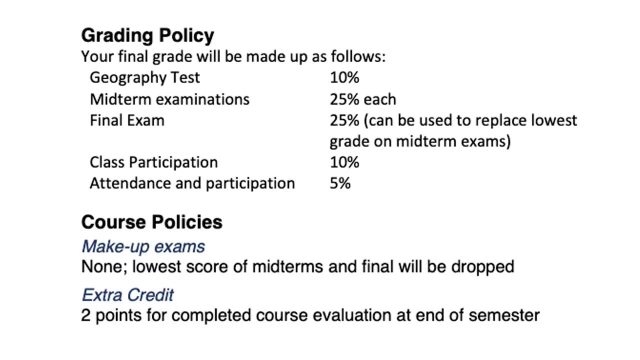 We correct the midterm quickly and go over right answers in the final class before reviewing what was covered in the course. Following the course review, a comprehensive final exam ends the class. Grades are based: 10% on the geography test, 25% each on the best three of four test scores. 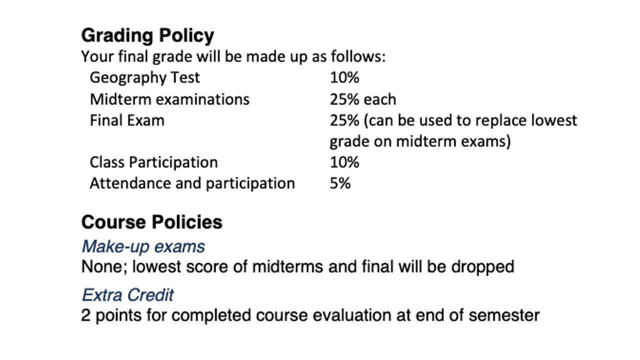 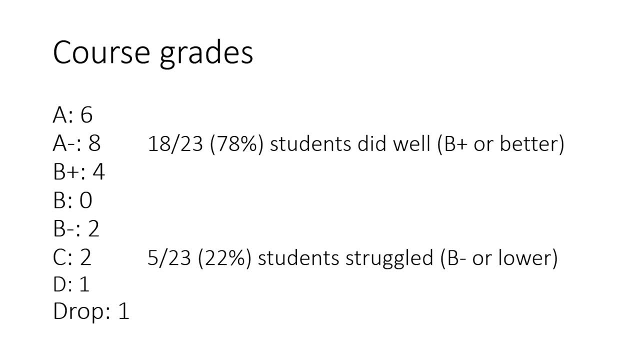 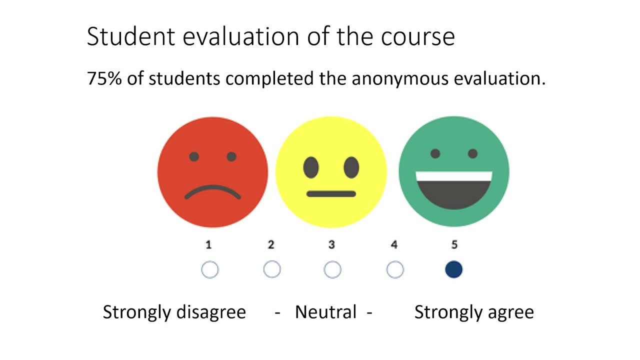 and 15% on class participation and attendance. Almost 80% of the students did well in the course, receiving a B plus or better. Only 22% struggled receiving a B minus or lower. We were especially interested to get feedback from the students, so we offered two points extra credit if students 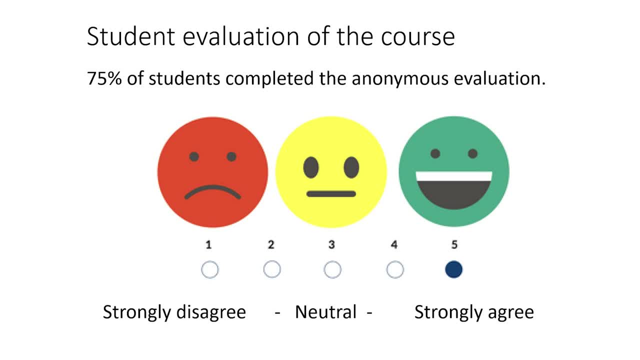 completed the UTD online course evaluation. We received 18 evaluations from the 23 students who finished the course. Mean evaluation scores ranged from 3.2 to 4.8 on the 5-point Likert scale, where a 5 indicates strong agreement and a 1 signals strong disagreement with each of 15 statements. 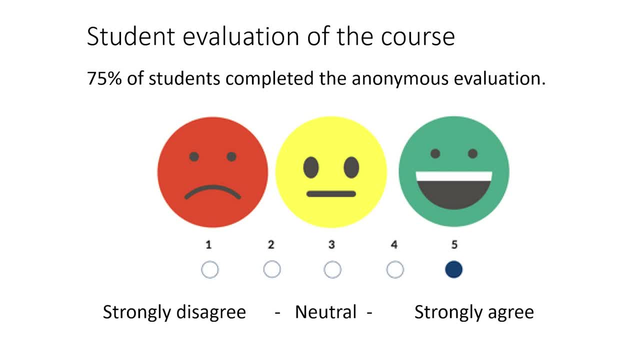 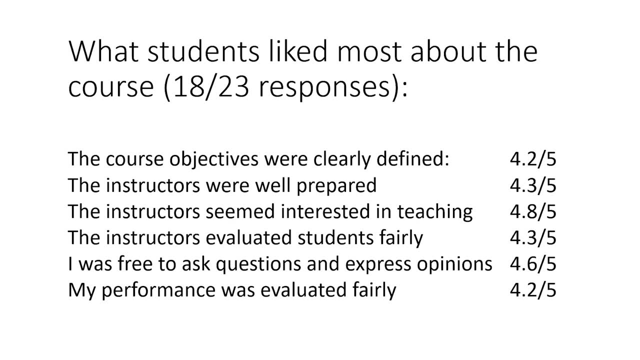 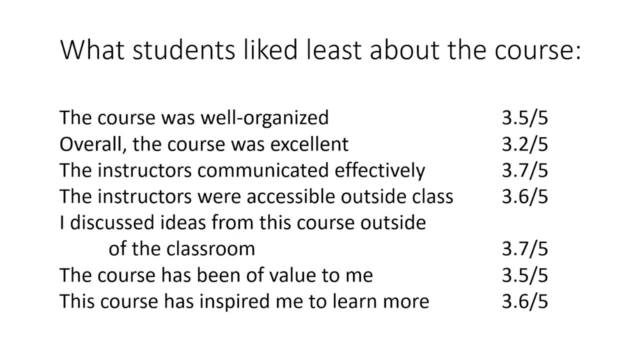 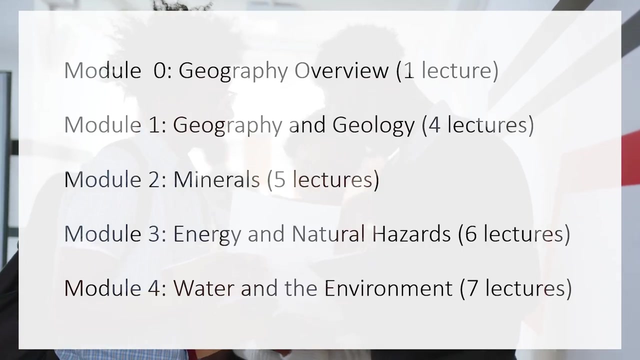 about the course. We received the best scores for course objectives, preparation, enthusiasm, fairness and encouraging student questions and opinions. We received the lowest scores for course organization, quality and value, and for our communications and accessibility. Overall, we are encouraged by student responses to the course. 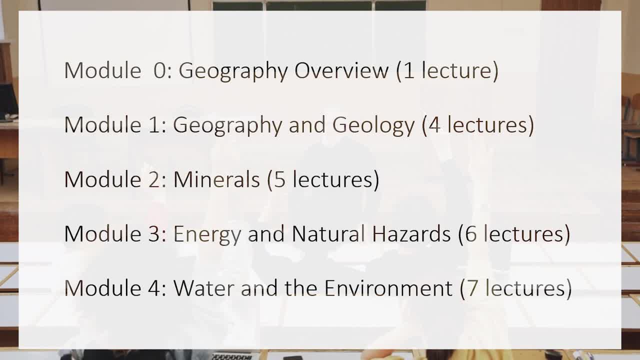 It is clear that the topic is important, the students are interested and that the course helps address the challenges of increasing diversity in science. It also is clear that we need to improve some aspects, which we intend to do. We will offer the course again in fall 2022 as a three-hour online course supplemented. 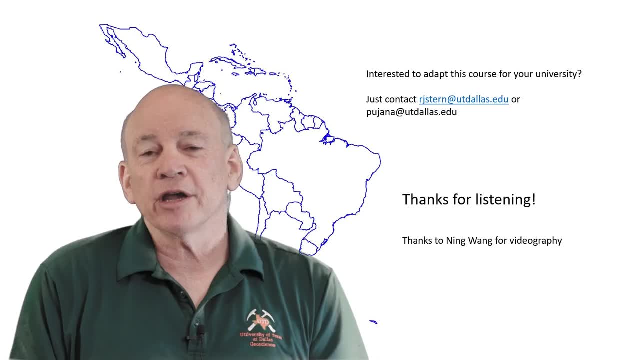 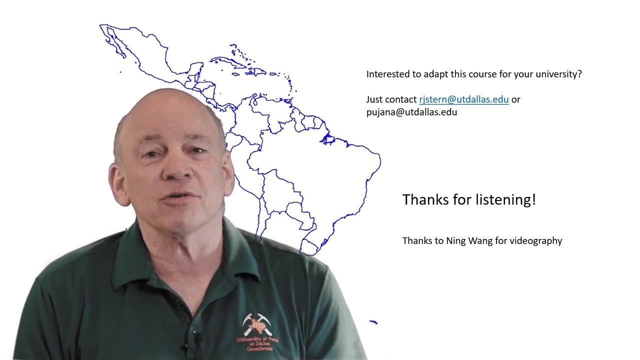 by a one-hour optional discussion course. We are happy to share course materials with instructors who would like to consider adapting it for their own purposes. Just email oneofusatutdedu. All we ask is that you share with us anything that you changed about the course, and any. 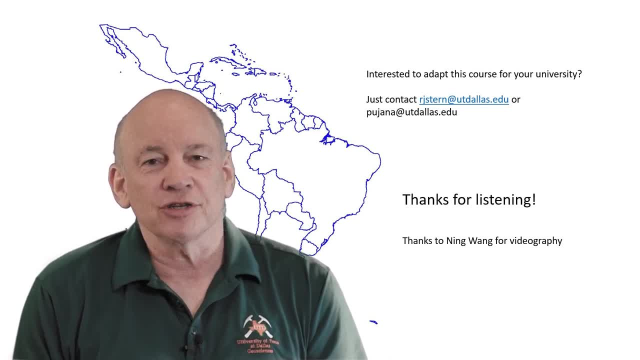 information, any feedback from how the students responded to your course. Thanks for your attention.